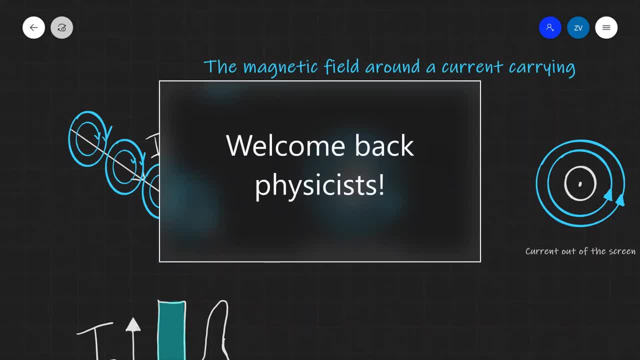 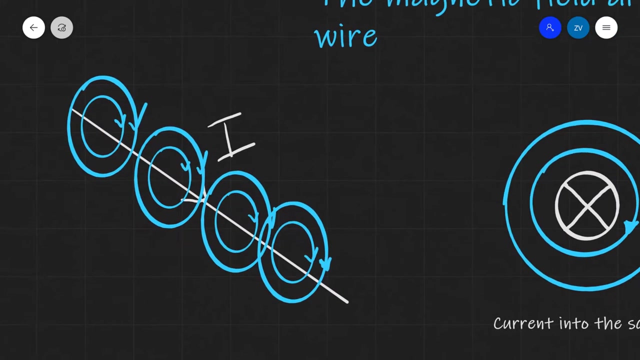 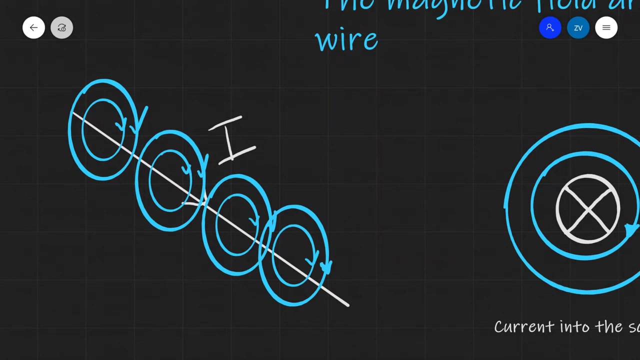 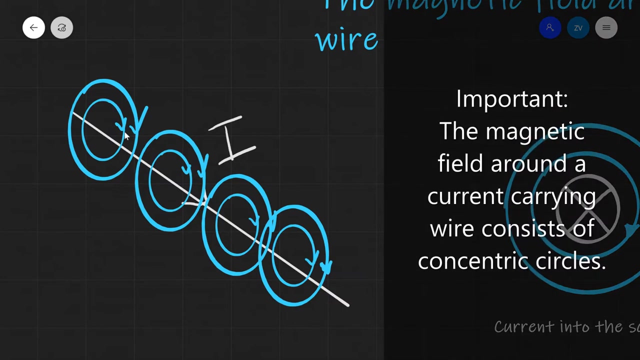 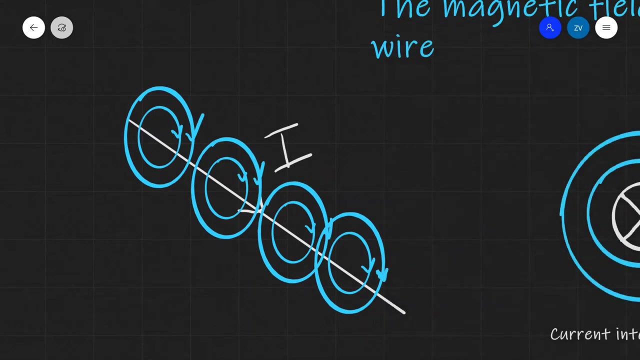 Hello guys, welcome back to Z-Physics. Today we're going to be talking about the magnetic field around a current carrying wire. This was actually one of the most interesting experiments in the 19th century which first probed the relationship between electricity and magnetism. Two seemingly unrelated phenomena which, as it turns out, would soon be unified into a single theory known as electromagnetism. What was first noticed was that magnets started behaving pretty strangely around the wire. In fact, you could essentially plot a magnetic field line simply by having a current carrying wire. We have this wire over here moving along with current i moving in this direction. If we were to probe the magnetic field around it with some magnets, and we do a plot, we'll soon discover that the magnetic field around the current carrying wire consists of concentric circles. Really really interesting. And those concentric circles are perpendicular to the plane at which the current is moving. One of the best ways to visualize this is with the following notation. Let's have a look at this notation. 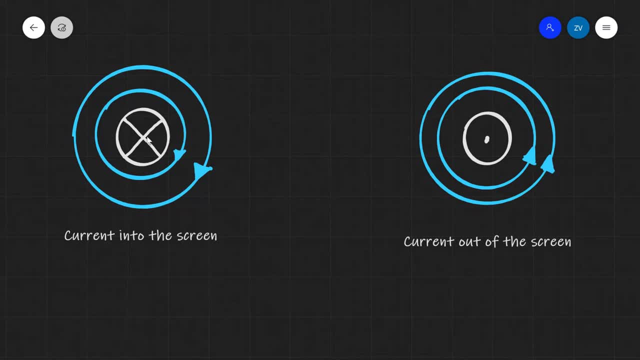 First off, now let's think in 3D at the moment, just like in the cinema. Oh wait, no, that's looking at 3D. But let's think in 3D right now. Imagine that this over here is the back of an arrow. So it's the back of an arrow that's been shot and it's going into the screen. 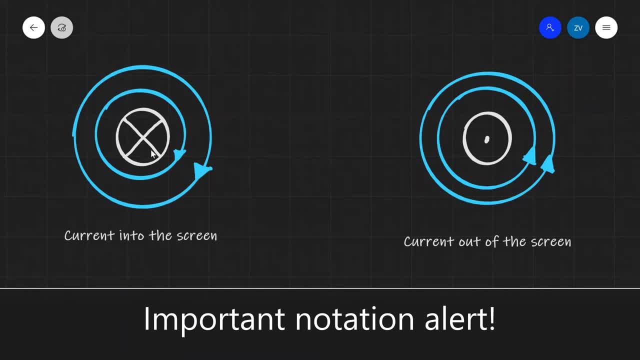 This is the convention for the direction into the screen or into the page on a test paper. Or into the board on a whiteboard in college, etc. And this over here is the tip of a arrow which is coming towards you. So in this case, this would indicate the direction out of the screen or out of the page or out of the whiteboard, etc. 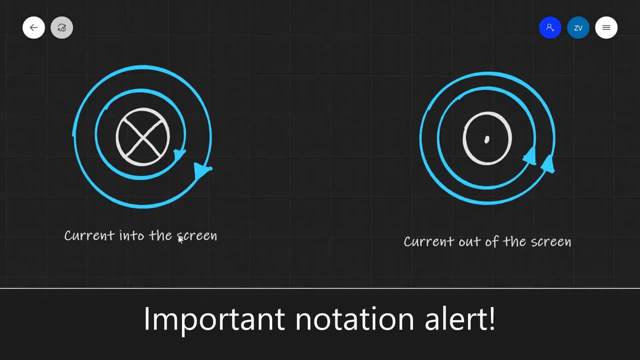 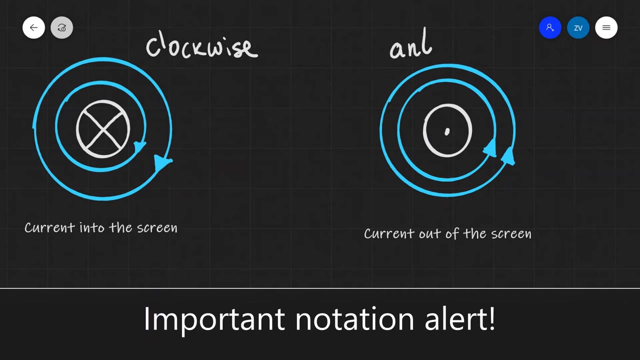 If we have a current carrying wire with which the current is going into the screen, we can see that the direction of the magnetic field will be clockwise. So this is a very useful fact to remember that the magnetic field is clockwise when the current is going into the screen. If it's going out of the screen, we can see that the magnetic field lines are going to be anti-clockwise like so. 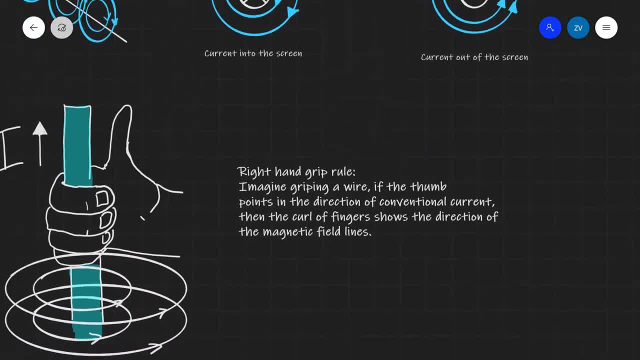 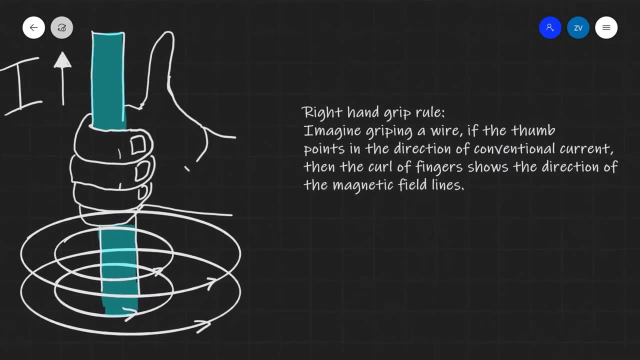 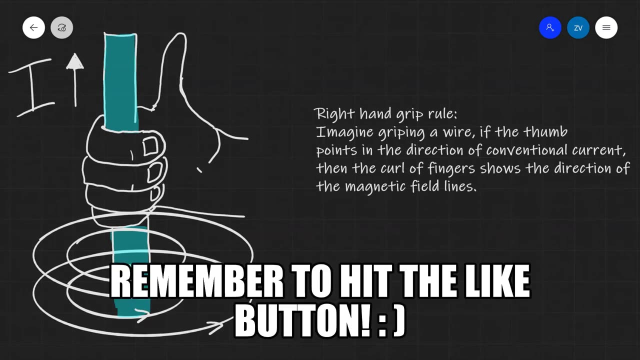 We can summarize this rule by the essentially the right hand grip rule which is an alternative way of trying to remember the same phenomena. You can see my little drawing over here with a thumbs up which just reminds me if you haven't liked this video, I think this over here is a good indicator to hit the like button. 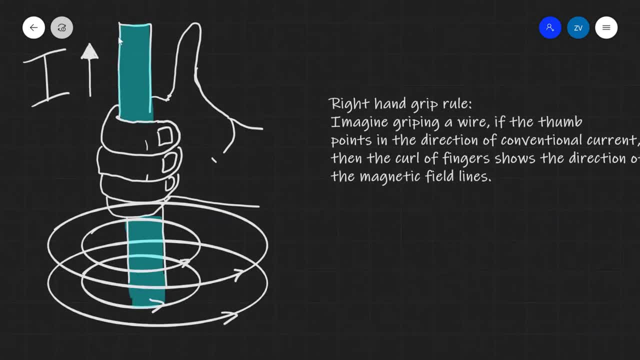 Now, looking at the current carrying wire, we can see that the current is going upwards. What we can always imagine to do if we have the direction of a current, imagine gripping a wire and align the thumb with the direction of the conventional current. Some exam questions may try and trick you by giving you the electron flow direction, but of course, any function of the term current will be the opposite direction if that's the case. 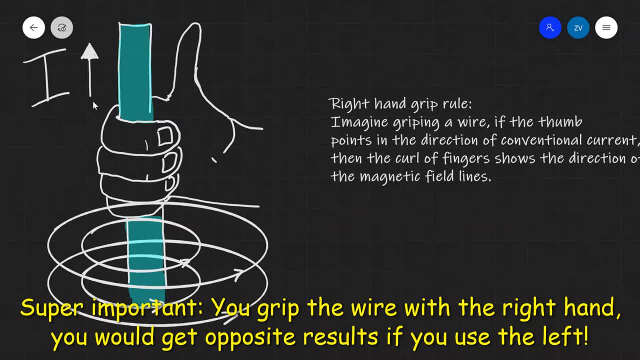 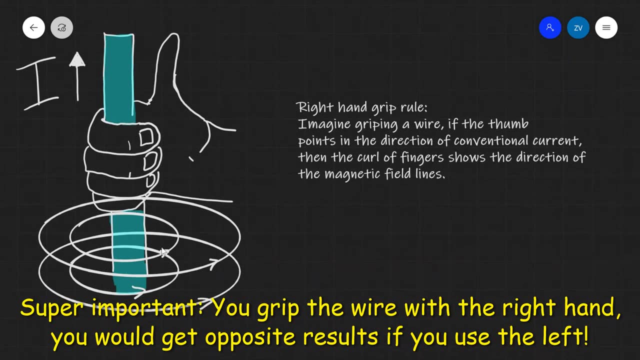 In either case, the direction of the conventional current is upwards. So, if we were to align our thumb with the direction of conventional current we can see that the curl of the fingers will coincide with the direction of the magnetic field lines. 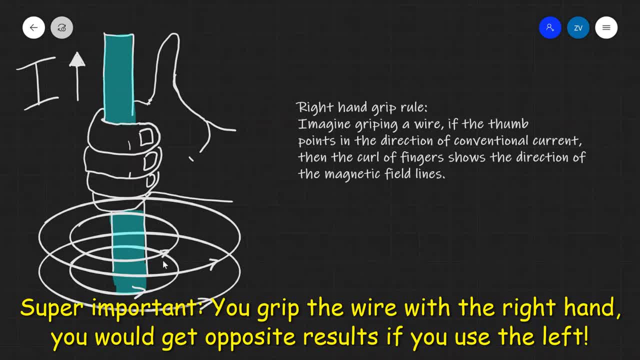 And we can use this as another way of remembering the rule for drawing magnetic field lines around a current carrying wire. 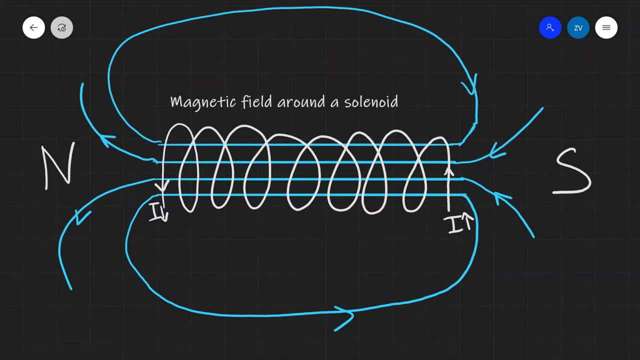 One more field I would like to have a look at in this online lesson is the magnetic field around a solenoid. Now a solenoid is just a fancy word for a loop of wire. And often there are multiple loops of wire. So we have a wire over here and we can see that we've looped this quite a few times. Normally there is a base and a core to a solenoid, but in this case it's just a wire that has been looped. 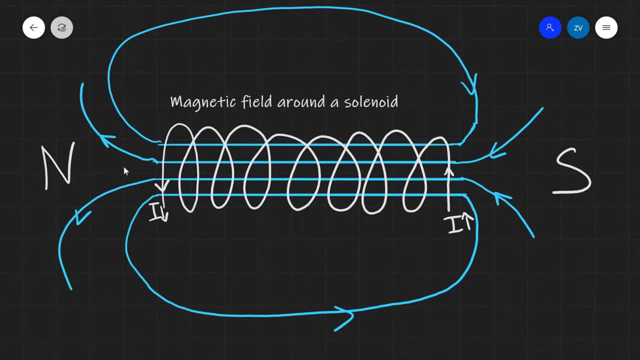 We can use the right hand grip rule to actually determine the direction of the magnetic field and plot a field around it, which I've done like so, given the current is going in the direction. 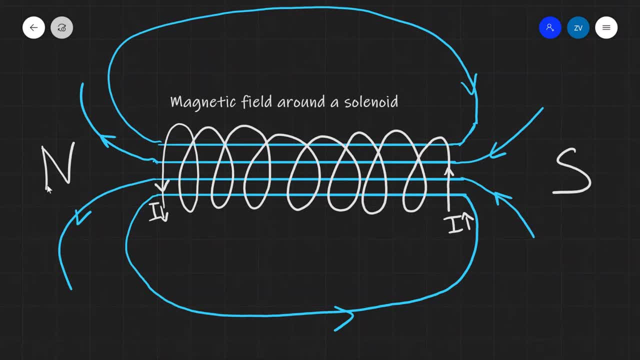 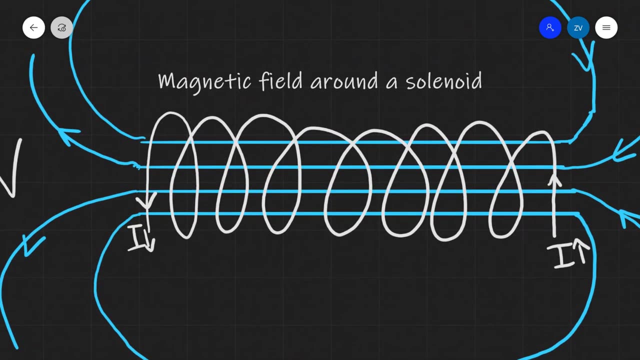 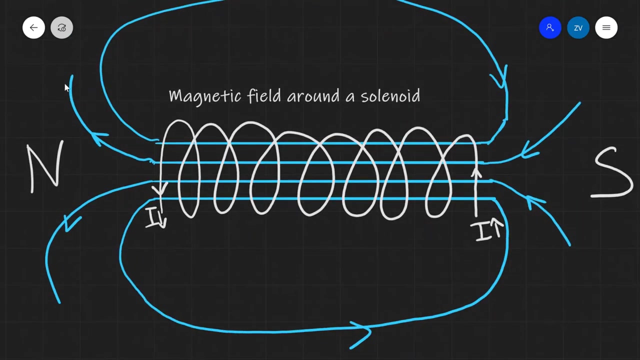 What we're going to find out if we were to do that is that the field inside of the solenoid is actually uniform. So this is really, really important. It is one of the ways to produce a uniform magnetic field. It's not quite uniform around the edges. Well, it's not uniform around the edges, as you can see. 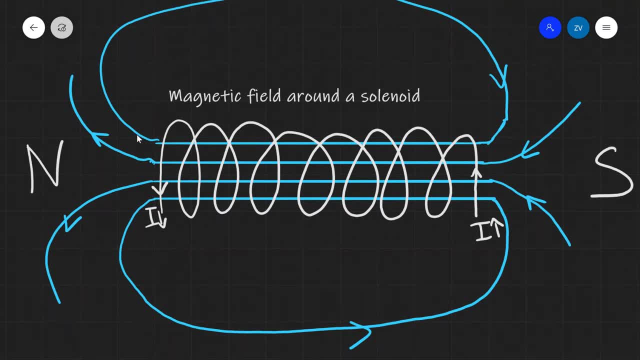 And the solenoid is going to act as if... it had a north pole and a south pole this is one way of essentially making an electromagnet simply by looping a wire and then running a current through it this will simulate the field around a bar magnet really really effectively and can be used for many many purposes in research and 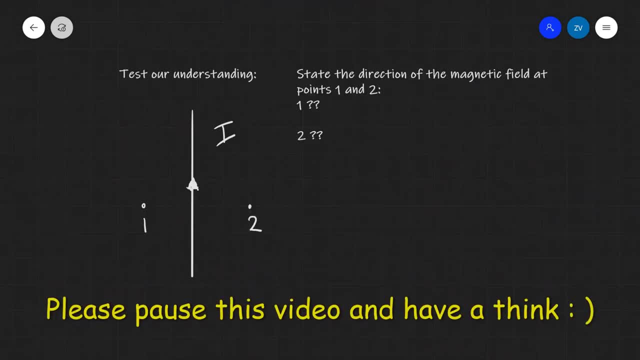 in engineering as well okay guys well let's finish off by testing our understanding we have a little question over here the we have a current carrying wire and the direction of the current is shown what what i want you to do is to state the direction of the magnetic field at the following points one and two so please go ahead and pause this video and have a think 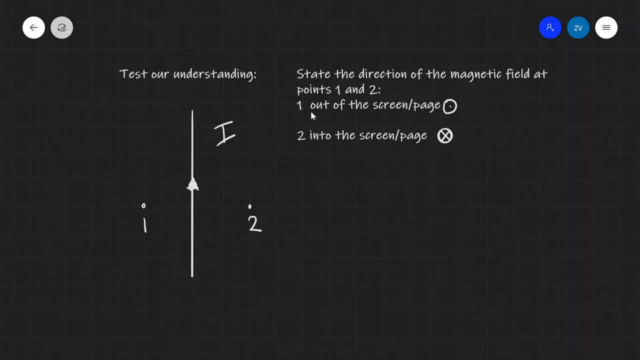 so the correct answer is that a point one the magnetic field is pointing out of the screen or out of the page of this was a test paper or if you're working on paper and at point two the direction of the field is into the screen or the page